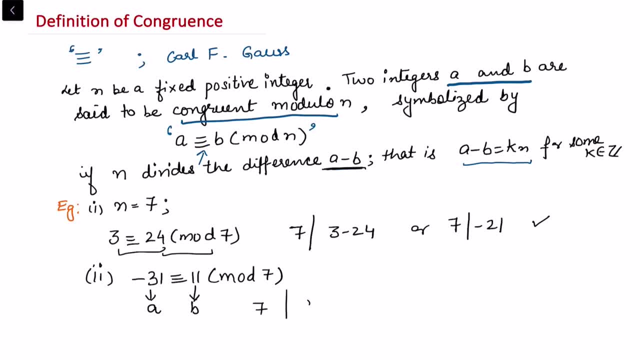 antithesis, And this is b. So we want 7 should divide a minus b. or I may say 7 should divide minus 31 minus 11, or 7 divides minus 42. So this is also true, because we say that 7, because we know that 7. 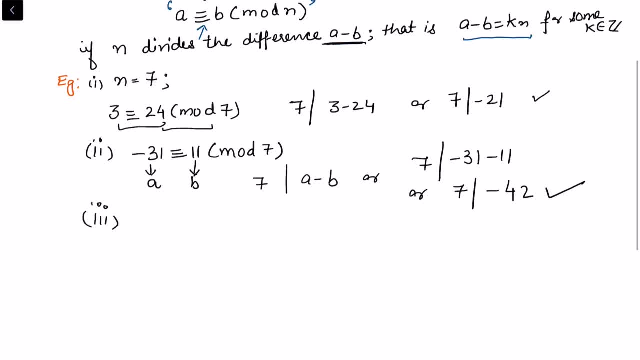 divides 42. So this means minus 31 is congruent to 11 modulo 7.. In another example I can take, minus 15 is congruent to minus 64 modulo 7.. Now in this case, what should hold 7 must divide minus. 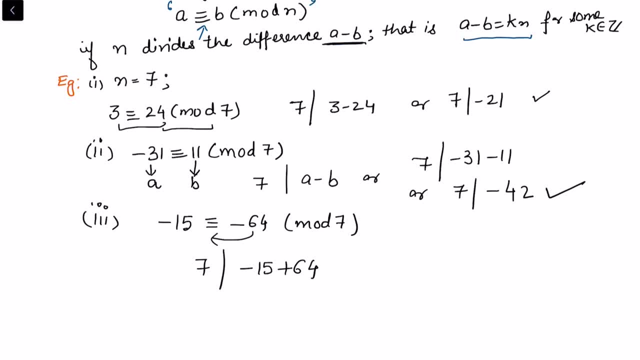 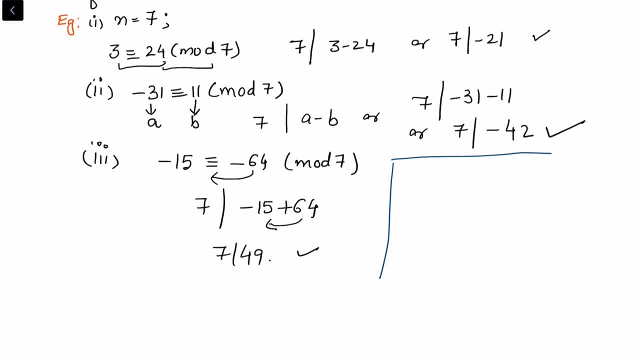 15. Plus 64. So taking this b on the other side, and that is why it is here with the plus sign. So this means 7 divides 49, and that is also true. So this way we can say that a is congruent to b modulo n. 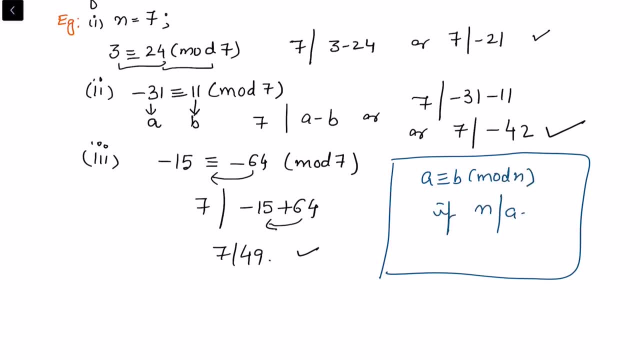 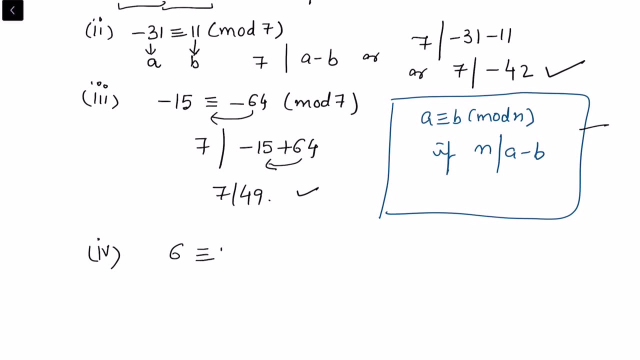 This has a meaning if n divides a minus b. So now consider some example in which this congruent definition is not satisfied. So suppose, I take, 6 is congruent to 1 modulo 3.. Now you can see that this is not true, because 3 does not mean that b is congruent to b. So this way we can say that b is. 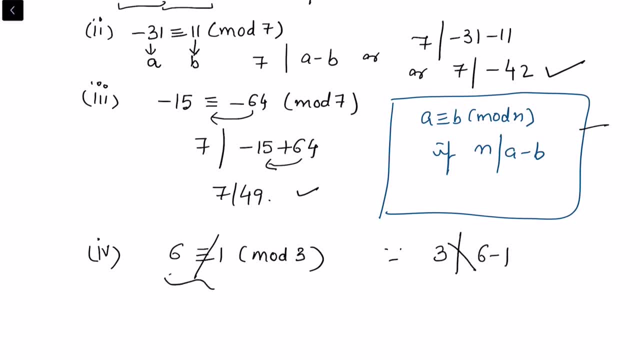 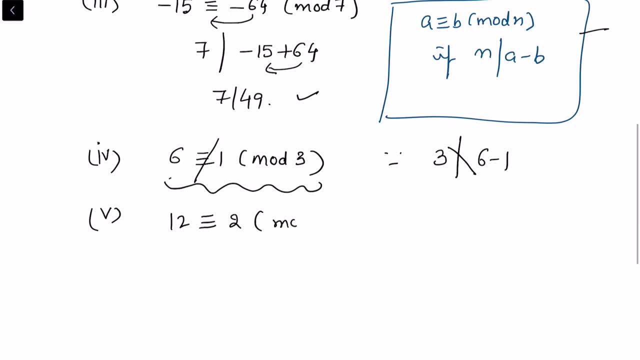 not divide 6 minus 1.. This is not true. So that means this congruent does not hold. And similarly- let us take some more example, I will take- 12 is congruent to 2 modulo 7.. This is also not true. 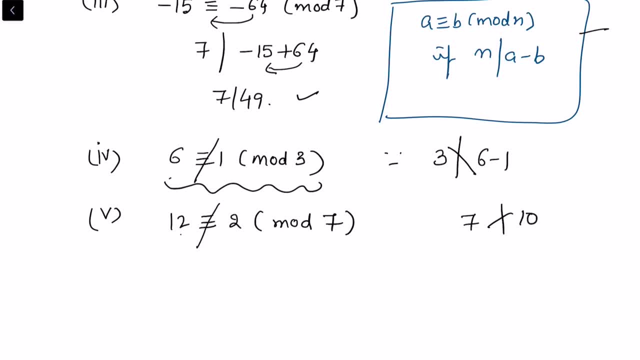 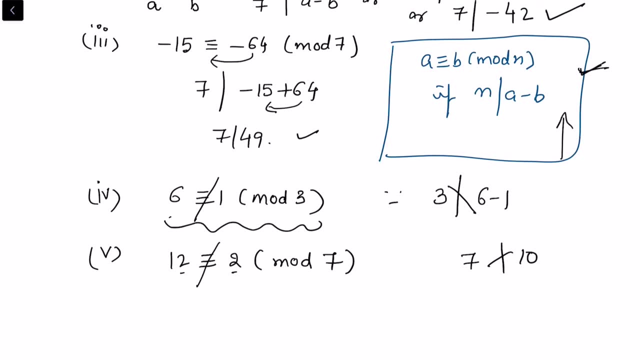 because 7 does not divide 10.. That is 12 minus 2.. So this way the definition of the congruent is actually the another way of writing the definition of the divisibility. Let's write some of the obvious remark and we can say that any two integers are congruent to b. So this way we can say that. 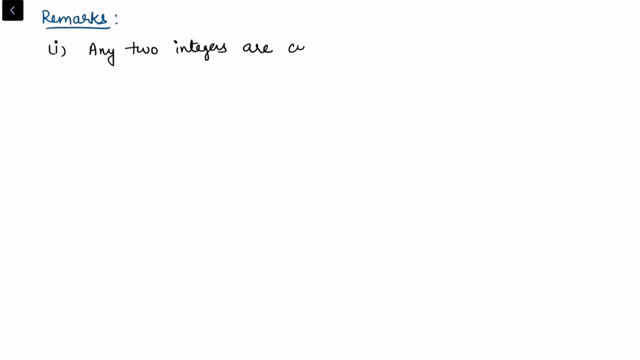 any two integers are congruent to b. So this way we can say that any two integers are congruent to b, So congruent modulo 1, because 1 will divide every integer, so we can say that any two integers are congruent modulo 1. so that means my expression, which is: a is congruent to b, modulo 1 is always. 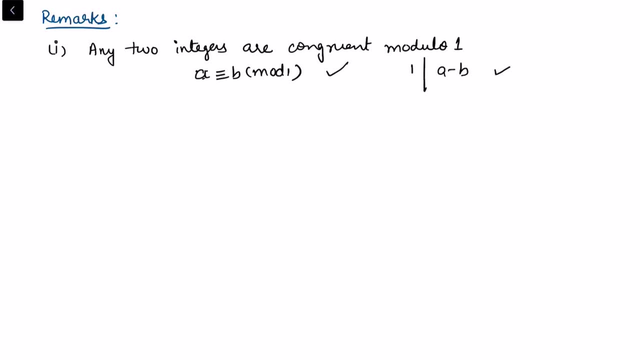 true. so this will always hold because 1 divides a minus b always. so that is always true. and second mark says that two integers are congruent modulo 2 if they both are even or they both are odd. so now, as we know that 1 always divide a minus b, so this was a very trivial case and to understand. 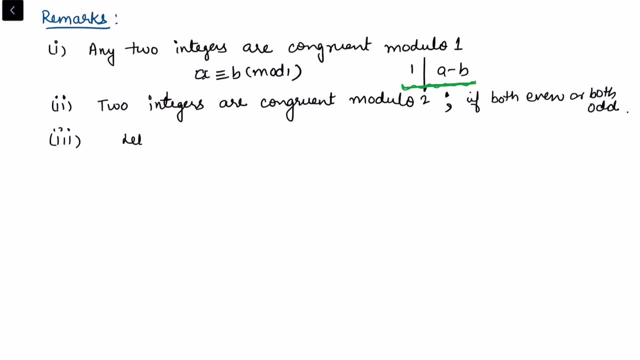 now in general, the congruences. let us fix an integer which is strictly greater than 1, and this will give us a non-trivial case. and now i am also using the division algorithm. so here i mentioned now by division algorithm now, and we also consider a integer, a. so consider an integer. 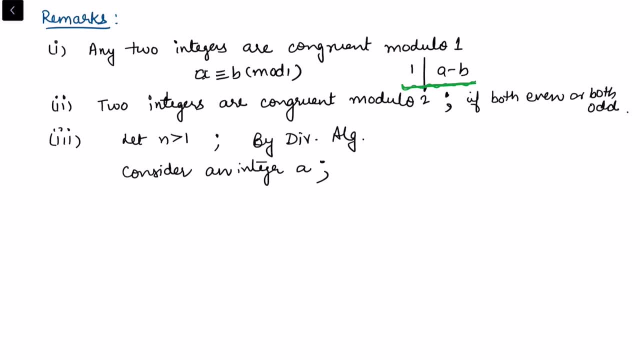 a and upon division this a by n. so we apply division algorithm. this will give me an expression: a is equal to q, n plus r. so this means there exists some quotient and remainder which satisfy this relation, and the remainder lies between zeros less than or equal to r, strictly less than n. now, looking at this general expression constructed by division: 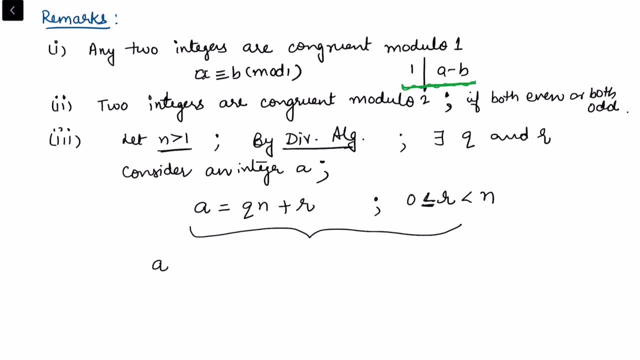 algorithm, and that is true for every integer. we can write a corresponding congruent. so this means a minus r is equal to q n, and that means this will now act as a minus b is equal to multiple of something. so i can always write: a is congruent to r modulo n, and here we know this will act as: 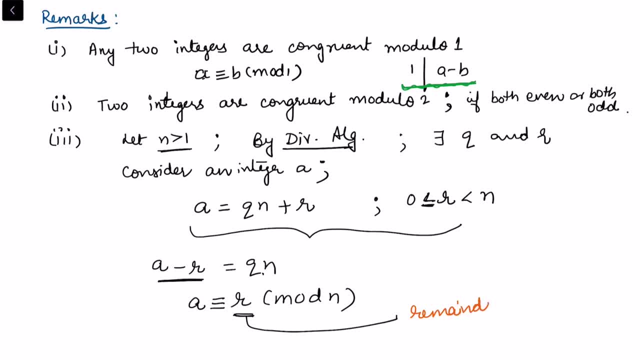 a and this will give us a. this is what is our remainder and if we go back to the previous definition of the congress, we have written: a is congruent to b modulo n whenever n divides a minus b. or i can say that a minus b is a multiple of n, because if n divides, this then means a minus b is. 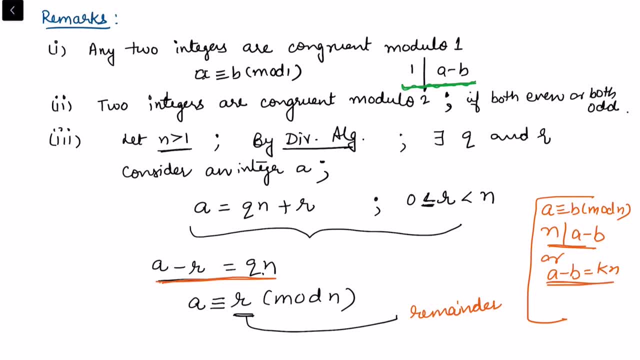 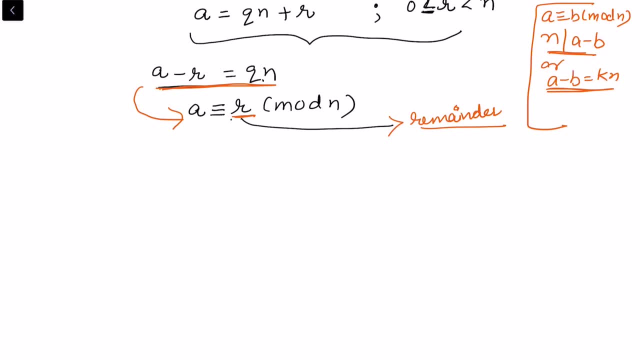 multiple. so from this definition and looking at this expression, i can now write this as: a is congruent to r modulo n, and this r is a remainder. here and now, if you want to see what is the possible values of this9534 and if you want to see what is the possible values of this9534, 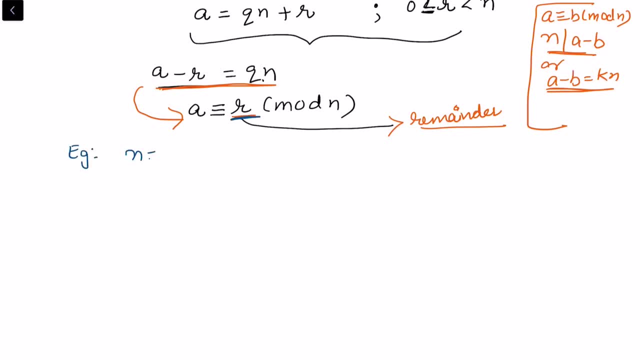 far. so for example, let's take it first in the example- suppose if n is equal to 2 and you take any integer a which is equal to r modulo 2. so we know whenever we divide any integer a by this 2. so the possibility for the remainder is either 0 or 1. either it is an even number or it is an odd. 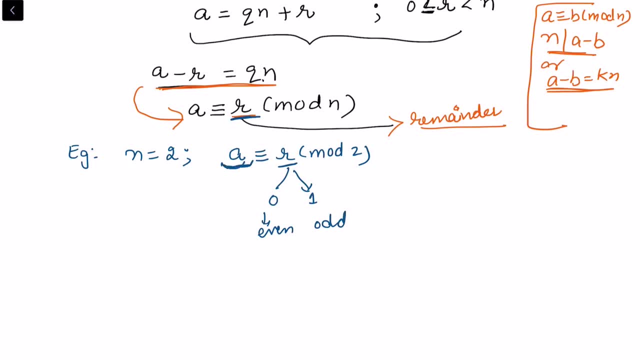 number. so this means for any a. whenever we divide it by 2, the possibility for the remainder is 0 and 1. so this means for r, the possible values are either 0 or 1, and similarly for n is equal to 3. if you want to see now what is the possibility for a, either it is 0 or it can be 1 or the remainder.